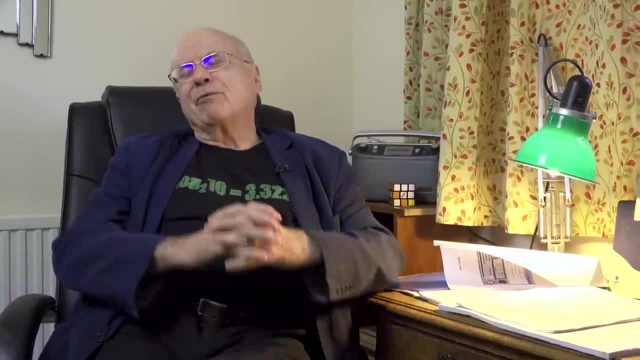 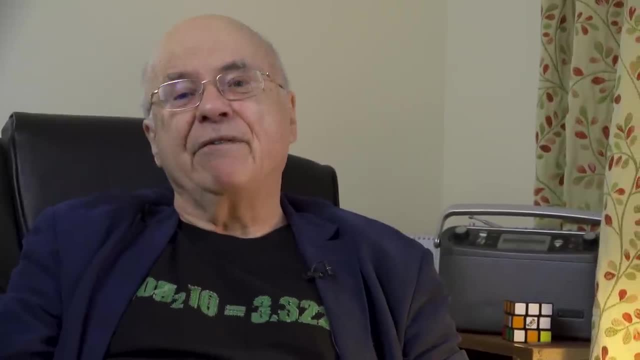 Neumann, and why is he mentioned alongside Turing? Well, right at the outset, let's say John von Neumann was the great-aunt, And if he was the great-aunt, then who on earth was John von Neumann? John von Neumann was the impossibly talented, impossibly charismatic, very wealthy uncle to. 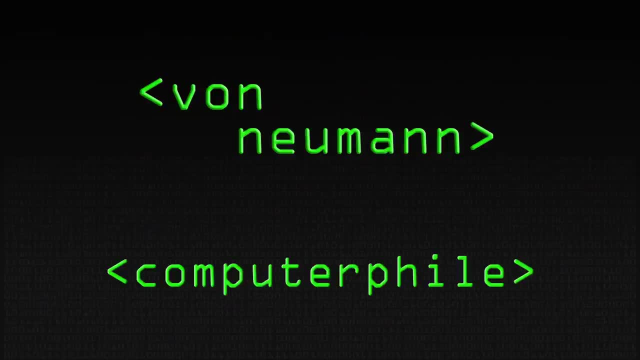 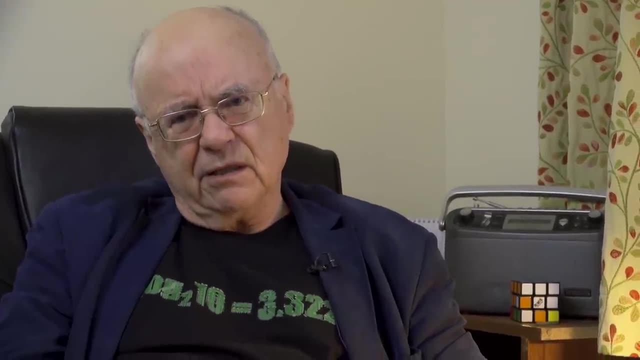 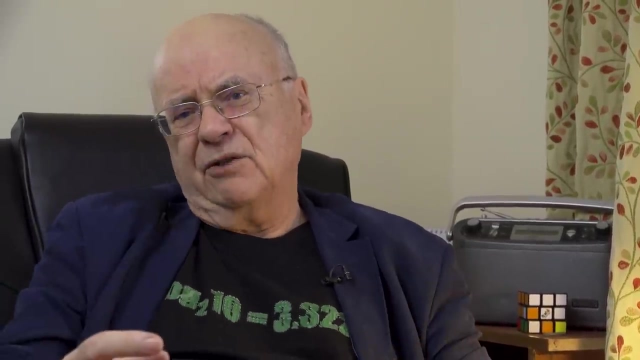 computing. It was he that, in the mid-1940s, in a way made it all happen by the force of his own personality and kept it not just in an enclosed community but encouraged all those who wanted to build general-purpose computers to come along to this summer school and do it. 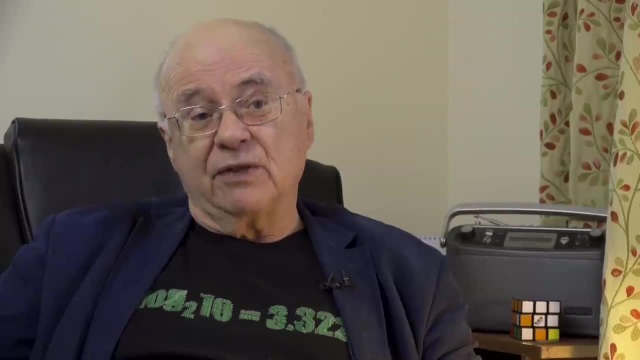 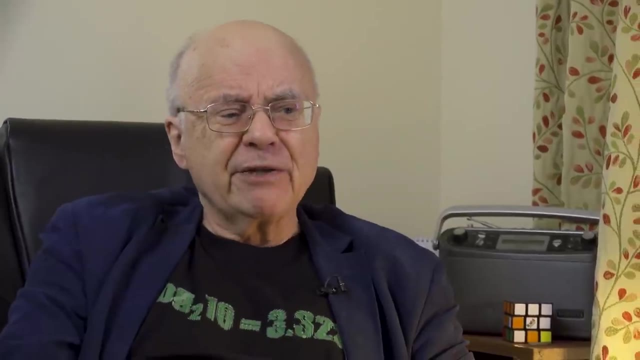 But that really I guess is in the future. It's where we've got to get to in the von Neumann story. But yes, you're quite right, Sean, to say that one of the first phrases, that almost any computer. 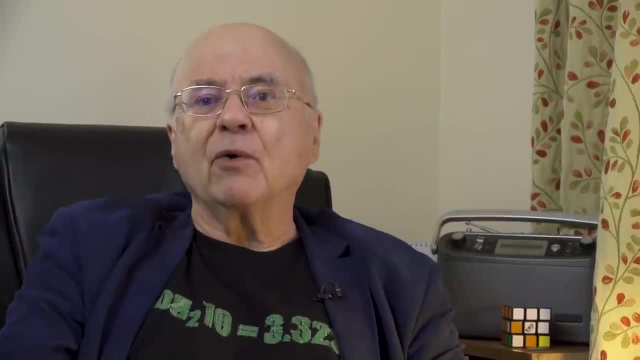 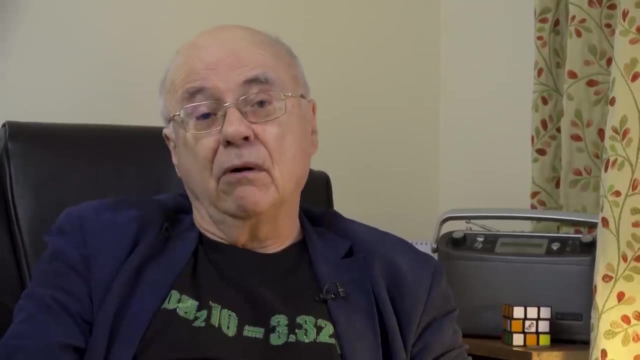 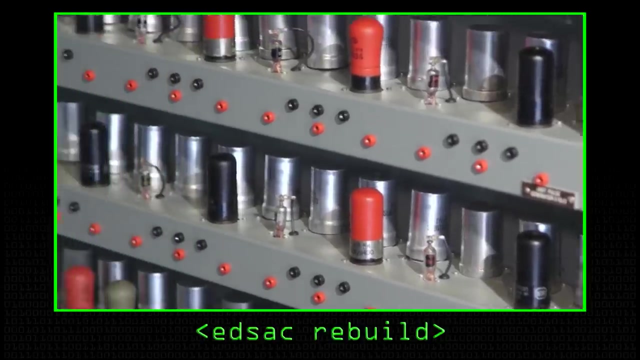 scientist hears about is the von Neumann architecture for computers, which to a large extent we still follow even now. all of what 60, 70 years later. So we've mentioned EDSAC before. We'll be coming back to mention this very. 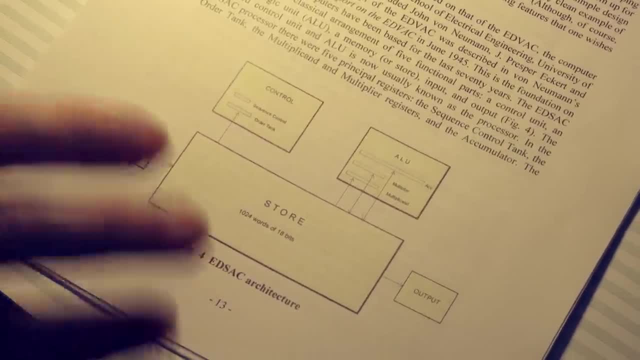 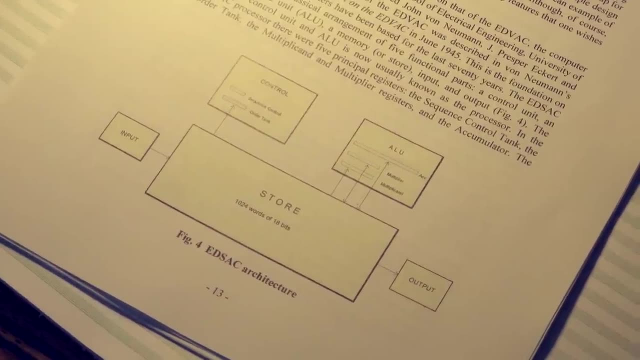 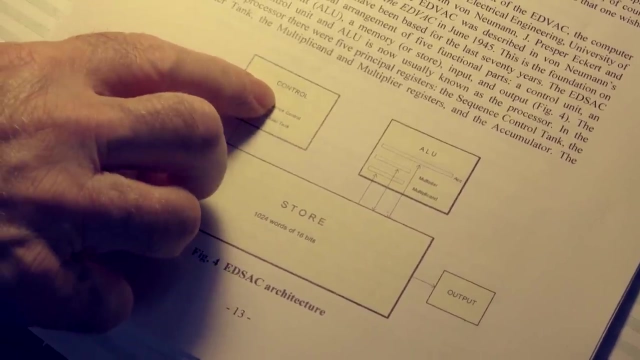 important early computer again, But it is a von Neumann machine and all it's saying is: it's very simple To build a computer. you need a store, or memory as it's more commonly called nowadays- to hold your instructions and your data. You need a control unit- often called a CPU now- and you need an arithmetic. 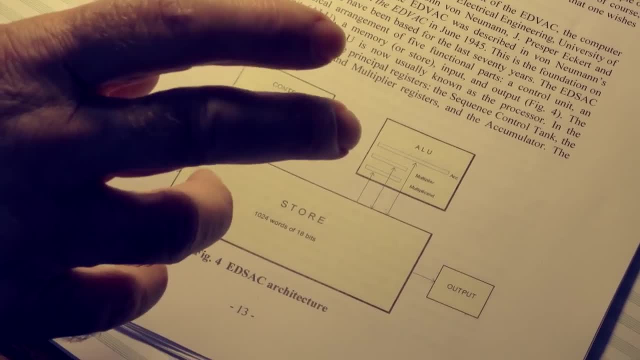 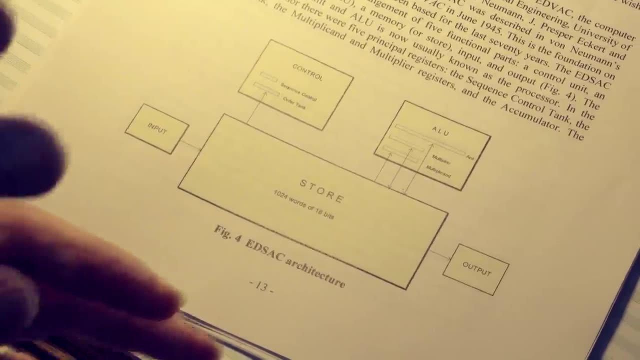 capability, the ALU, the arithmetic and logic unit. Again, many of you will know that in modern chips those two are often combined into what we just call the CPU chip nowadays, And you need input devices of various sorts, leading back to 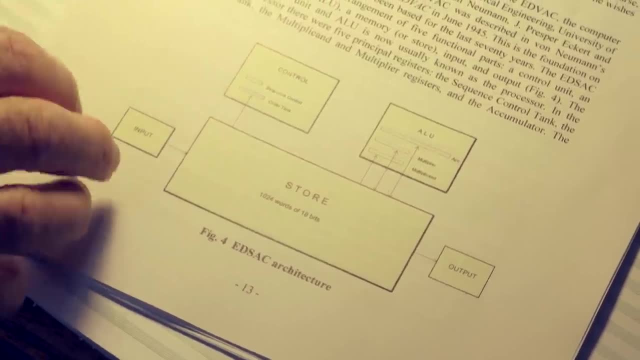 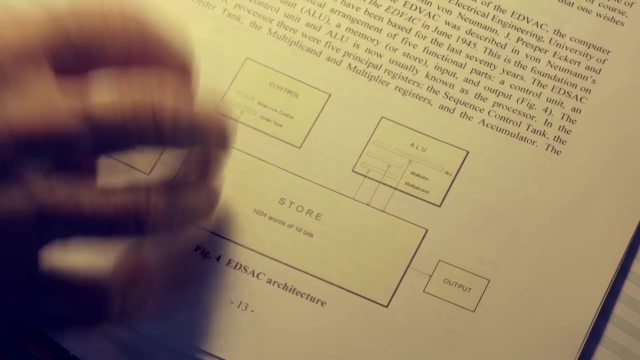 people's teletypes, input-output devices for backup storage disk and so on. You need to be able to do input and output. So there it is. It's just one, two, three, four, five boxes. That is the von Neumann architecture. 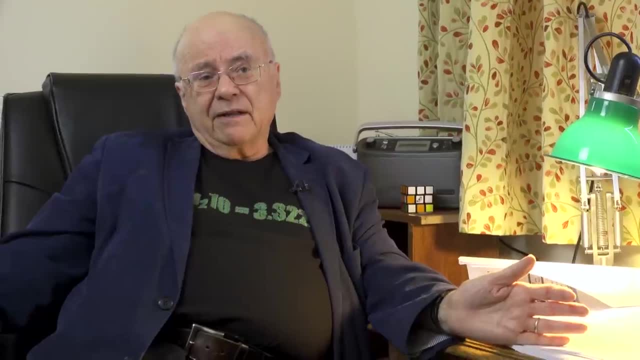 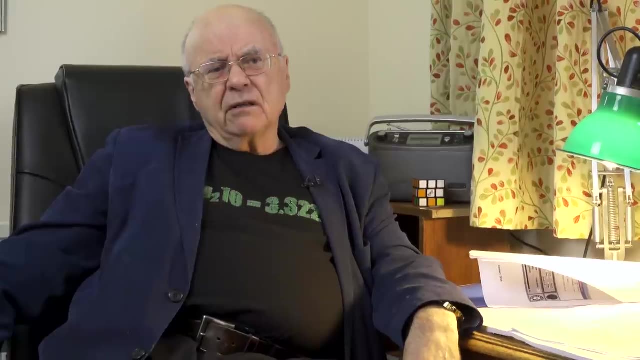 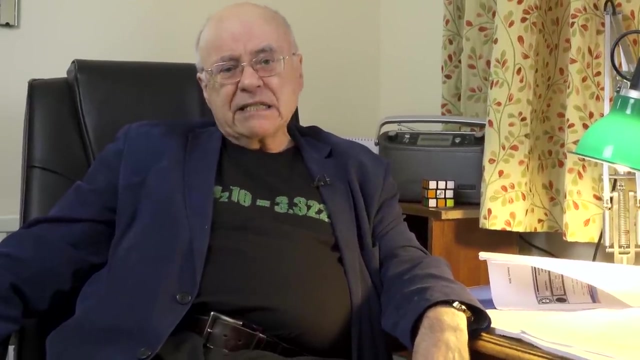 And it's very, very similar today. There was a big debate at the time about that store, that memory. Shouldn't you use it? Shouldn't you, for safety's sake, put the instructions of your program in a different sort of memory to your data? Wouldn't it be safer to do that? and 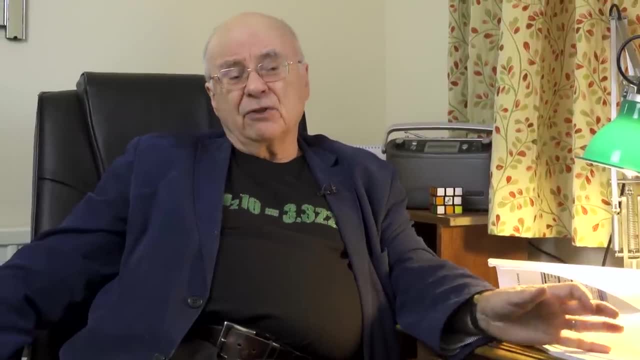 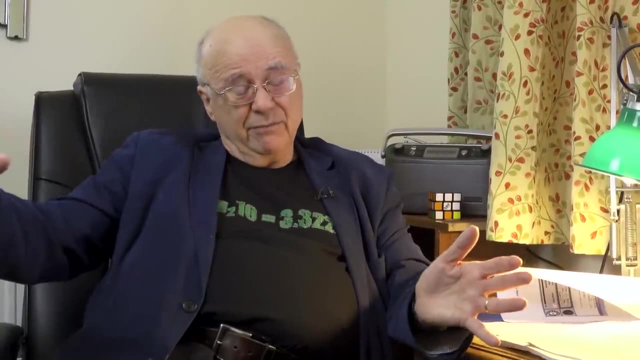 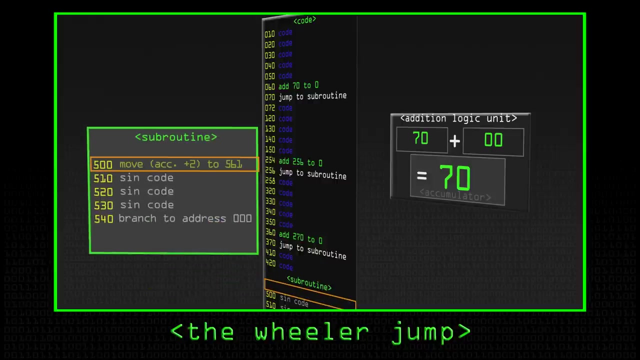 better in some ways. On the other hand, clearly if you've got a good memory technology that works, the temptation might be just to put them in separate areas of that same technology and try and take some sort of precaution about them not interfering with each other In EDSAC. the only way to get in the 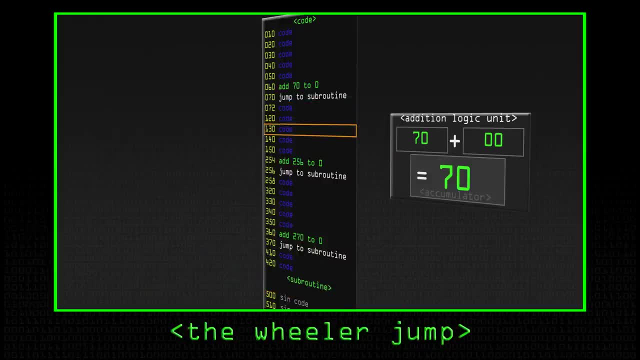 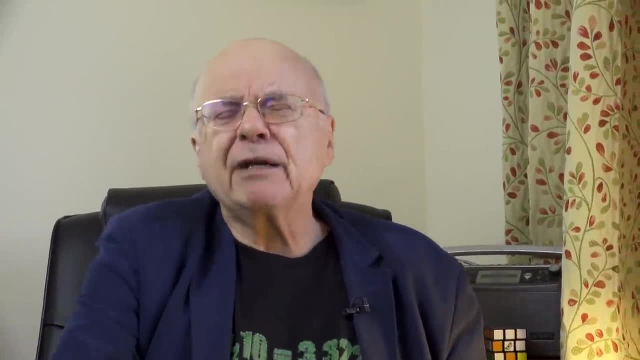 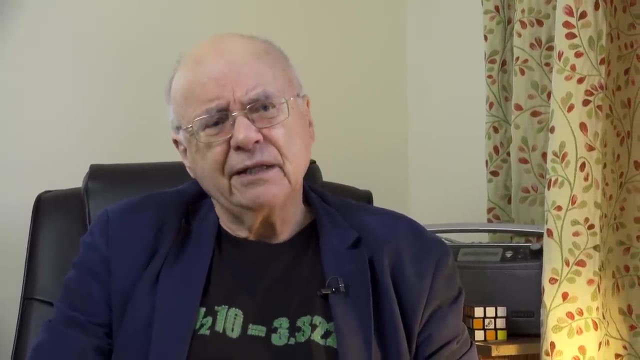 into a subroutine and get back out of it again was to override part of your program instructions. Let's just return back to this incredible character, John von Neumann. How does he fit in alongside Alan Turing? Well, like I said, he's the. 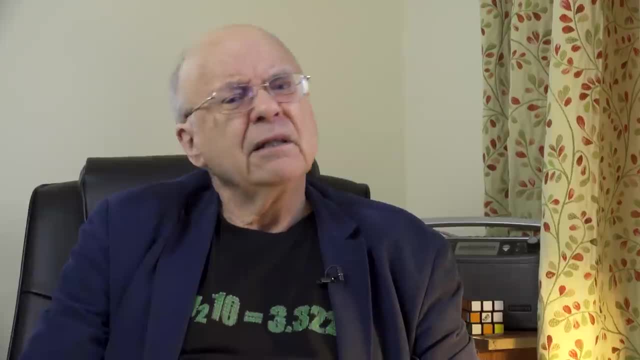 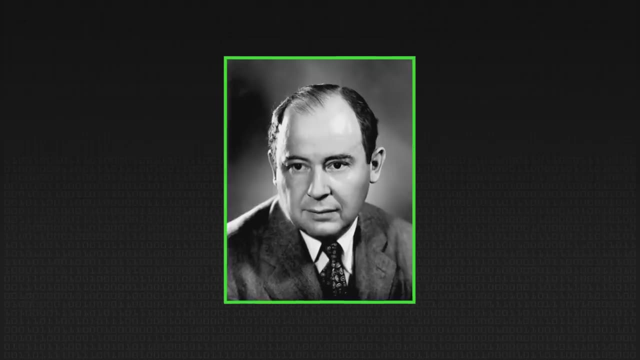 older, impossibly talented uncle. Did Turing and von Neumann know each other? Oh yes, they did. They were both basically trained as mathematicians. Von Neumann, It's hard to know where to go. It's hard to know where to begin and where to end. You can't exaggerate enough about how. 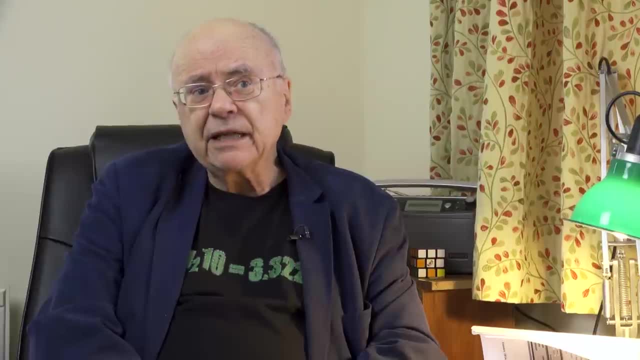 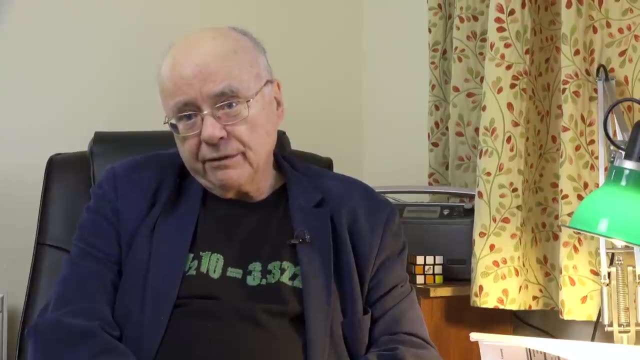 good he was. He was Hungarian and his Hungarian name, where they give surnames first, was, I think, Neumann Janos. His father was very, very wealthy and when von Neumann was quite young, the family became ennobled in Hungary, became. 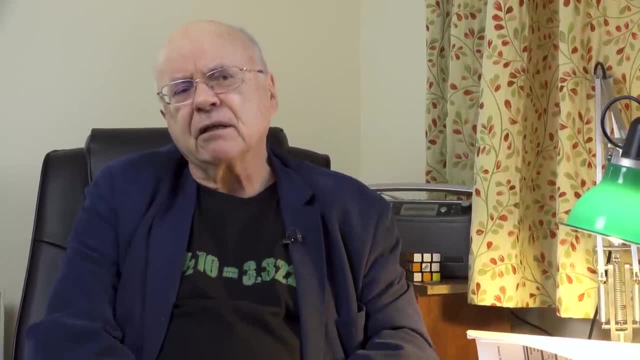 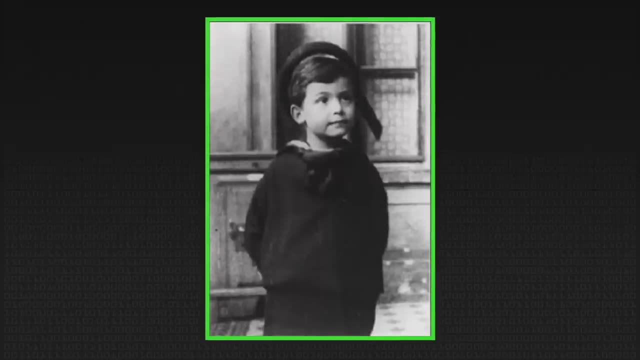 basically at the level of baron, hereditary baron, I think, over here. Janos was very talented. He was a childhood prodigy. He could divide wine eight-digit number by another eight-digit number in a fraction of a second, when he 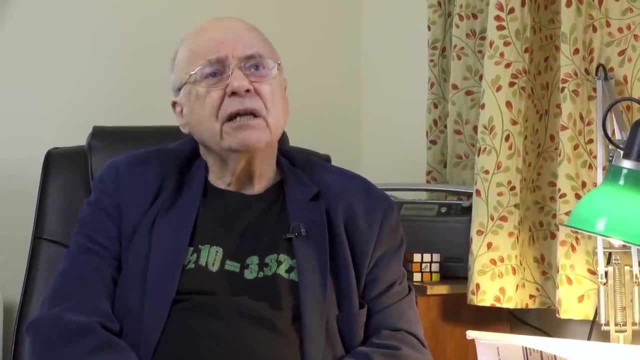 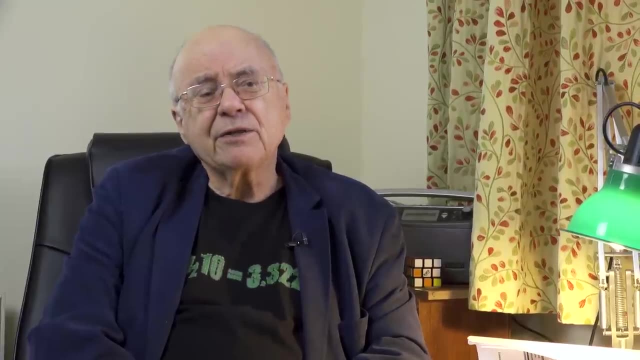 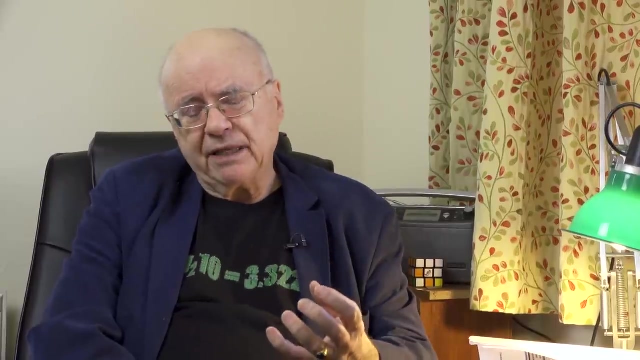 was aged about six. He loved history. He was a multi-talented polymath. He easily came top of the class. He effortlessly took in detail, and that's the first thing that all of his mathematics contemporaries said about him was his sheer speed at picking up new ideas and seeing the ramifications of them. So he 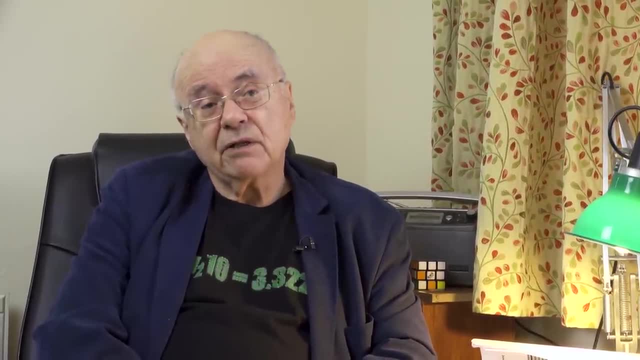 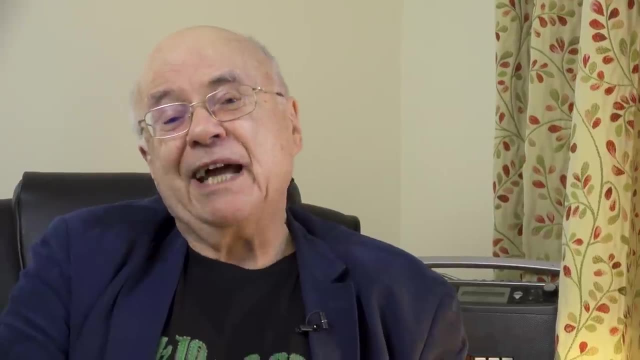 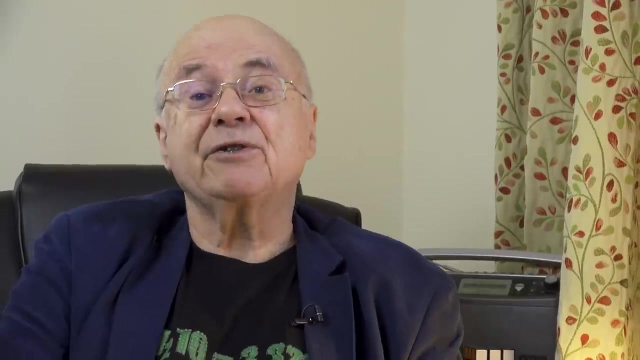 was notorious even as a teenager and as a maths undergrad He did his early education, I think, up to PhD level in Budapest. He almost naturally ended up at a place we've mentioned before in connection with Gödel and Hilbert- I'm talking, of course, about Göttingen University in Germany. 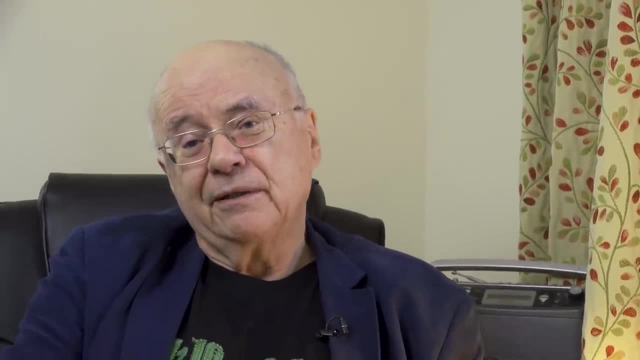 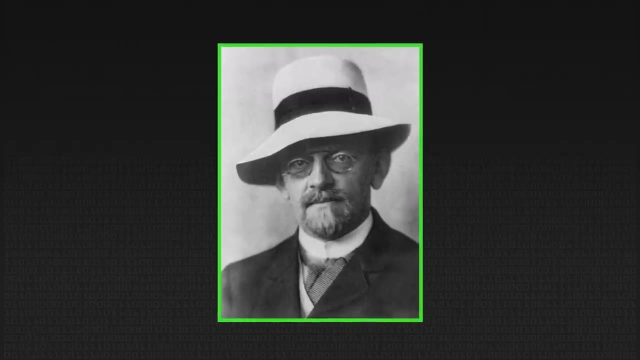 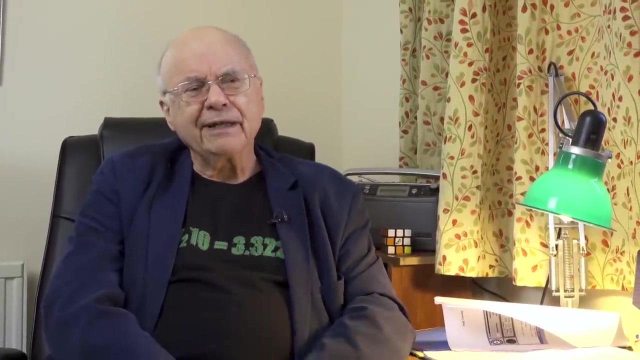 So Neumann Janos makes the journey via a PhD to becoming effectively the research assistant to the superstar David Hilbert at Göttingen. But because his family had been ennobled, he's not Janos Neumann anymore. Neumann Janosch, sorry, He's Johann von Neumann. 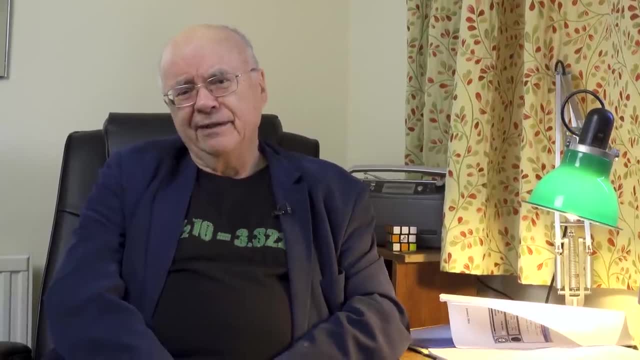 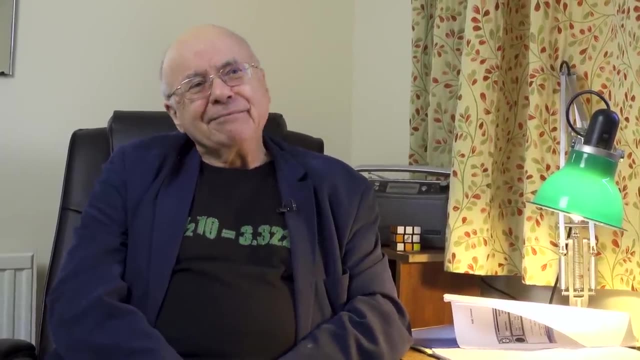 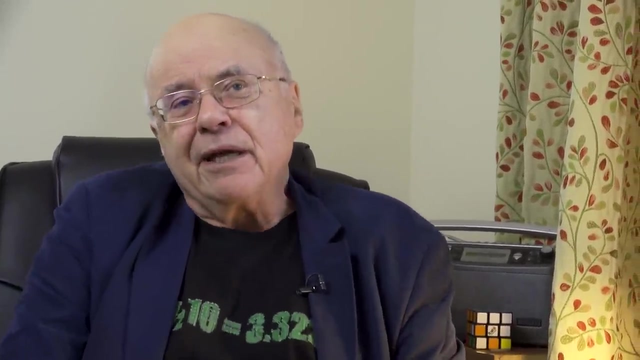 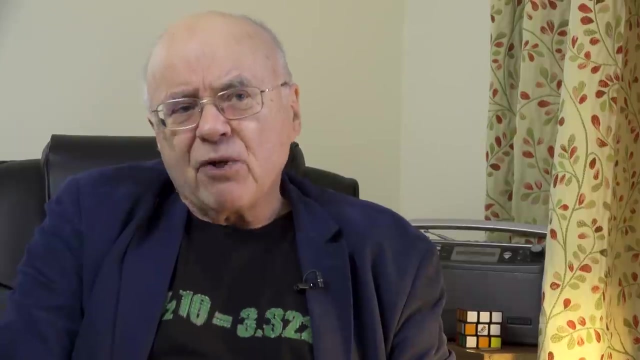 Impossibly talented Hilbert, his supervisor, at a seminar given by John, asked who his tailor was, because his impossibly smart pinstripe suit was just a complete knockout. So he was a legend almost the moment he got there and did some fabulously important work there. It was 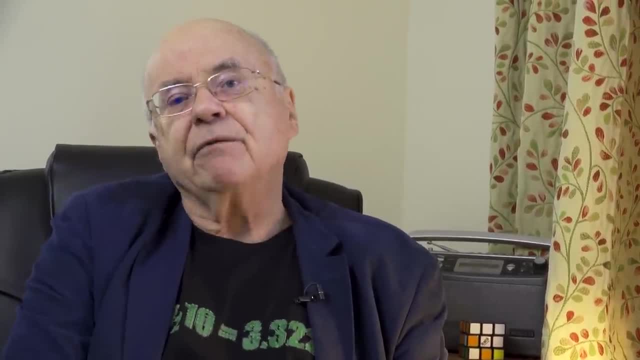 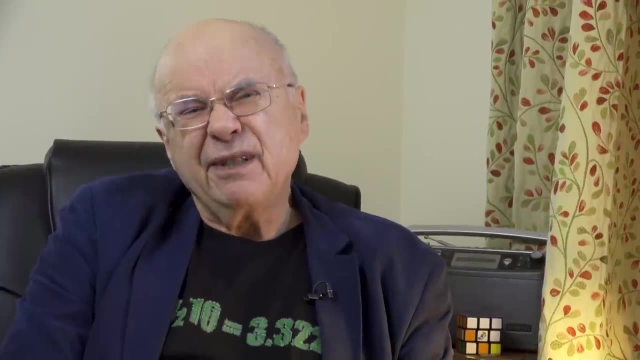 obvious that for somebody of his talents he was going to get a full professorship very quickly indeed. I think he became impatient of waiting for it to happen at any German university, So in the late 30s, 37,, 38,, somewhere around there anyway. 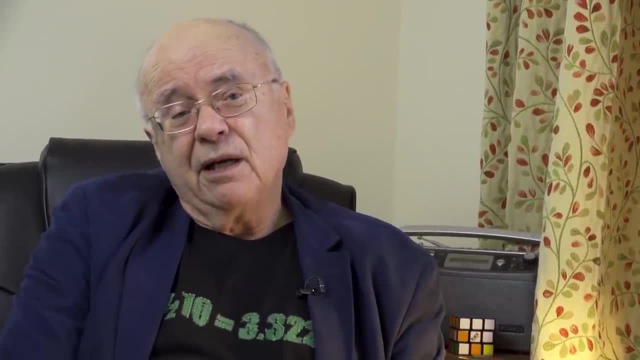 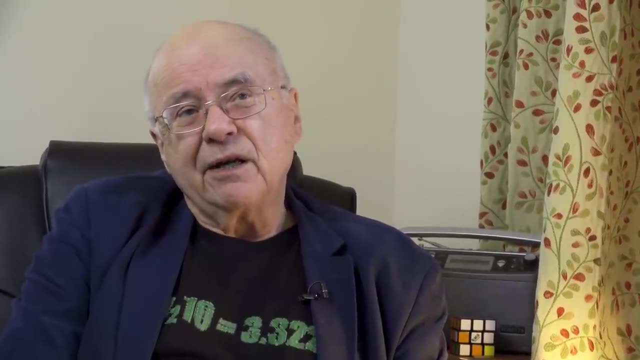 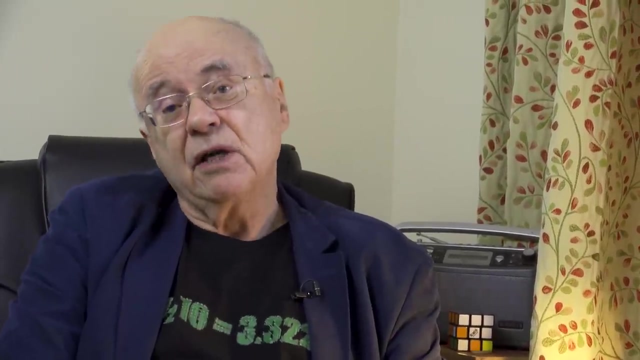 he got an offer from Princeton in New Jersey And that was, I don't know, very timely. It's all fitted in together very well. As part of his tours of Europe giving seminars and on his way to Princeton. I think he met Turing in the mid-30s in Cambridge because he gave seminars there. 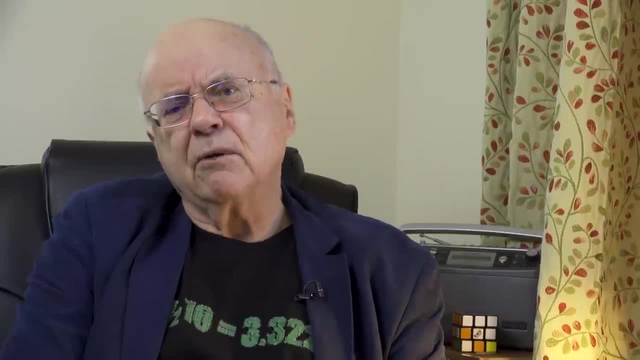 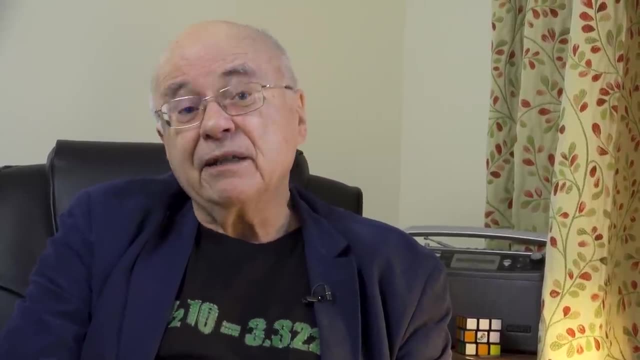 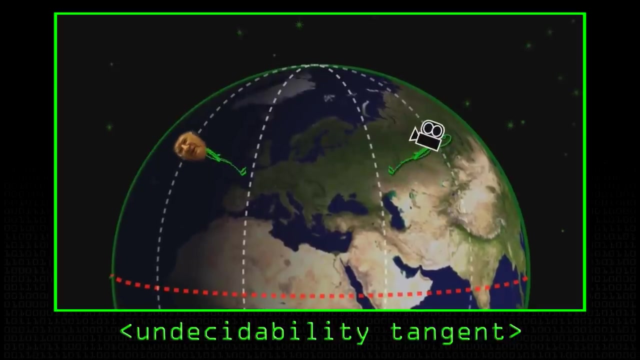 And I think a lot of mutual respect grew up. I mean, obviously Turing being in awe of von Neumann wouldn't be so exceptional, But after that 1936 paper of Turing's about decidability, following on from Gödel, and all that von Neumann, 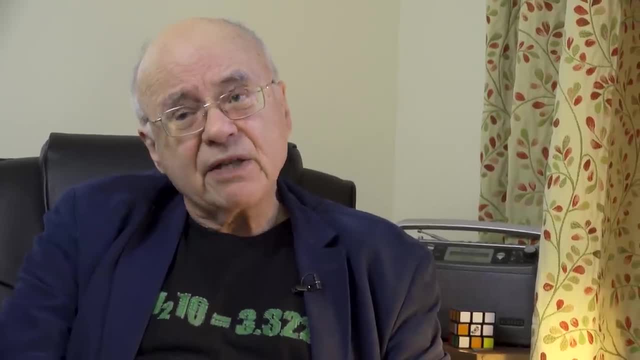 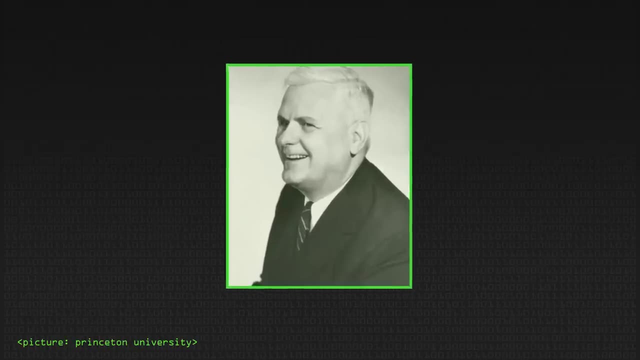 rated Turing. There's no question about that. This was evidenced by the fact- you will recall- those of you who've seen my previous videos- that Turing also took a sabbatical and worked with Alonzo Church at Princeton. Well, von Neumann was there by that time. Von Neumann was such 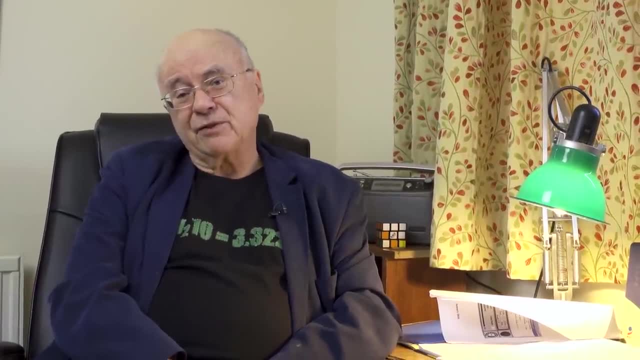 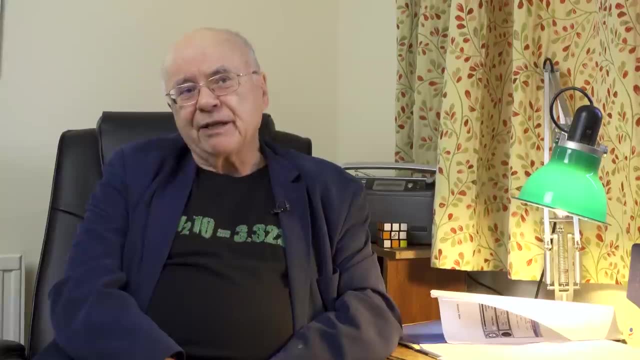 a superstar. They not only made him Professor of Mathematics at Princeton at an absurdly early age, probably about 30, something like that. but some of you will recall, right next door to Princeton, about a mile and a half across the meadows, is the Institute for Advanced Studies, which had been endowed in 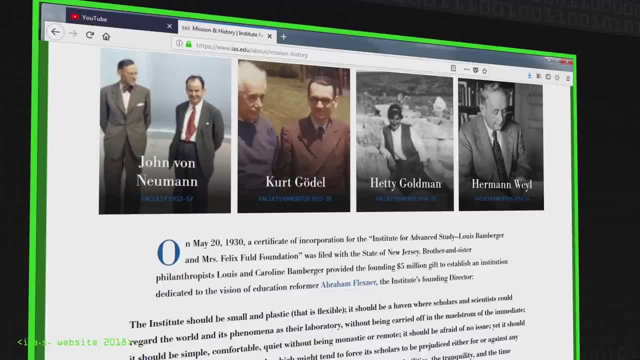 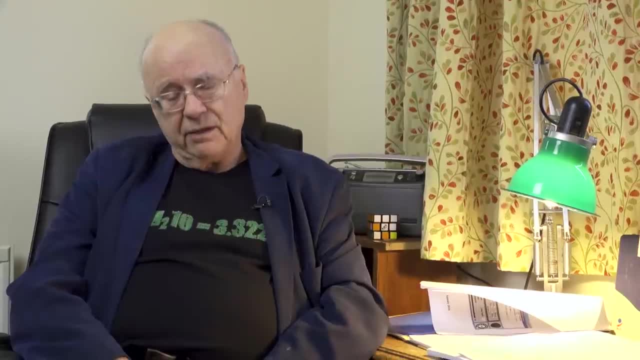 the early 1930s by a multi-millionaire, And this really was the ultimate club to be invited to join. You've got to be of the quality of Einstein, who accepted the invitation. Hermann Weyl, one of the founders of quantum mechanics, Gödel We. 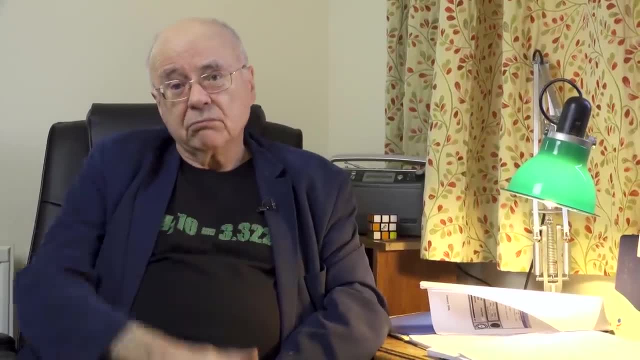 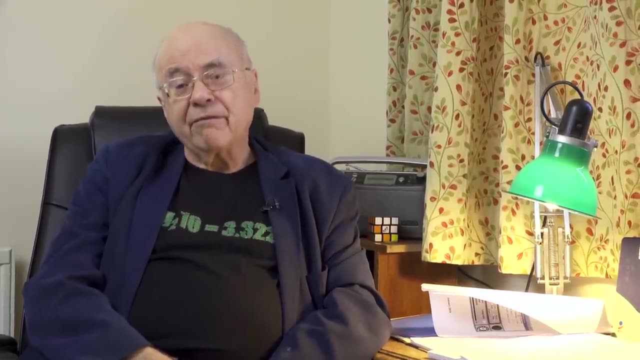 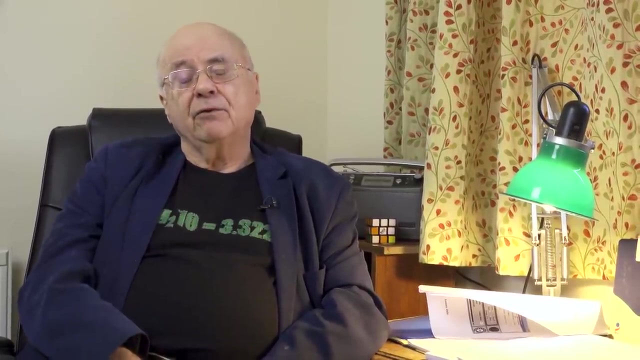 know about Gödel. Gödel was invited to just come to IAS Institute of Advanced Studies at Princeton. Stay as long as you like. Yes, you're a professor. Everything found, Food, accommodation, a lot. All we want is to have the greatest minds here. Von Neumann was offered a professorship in. 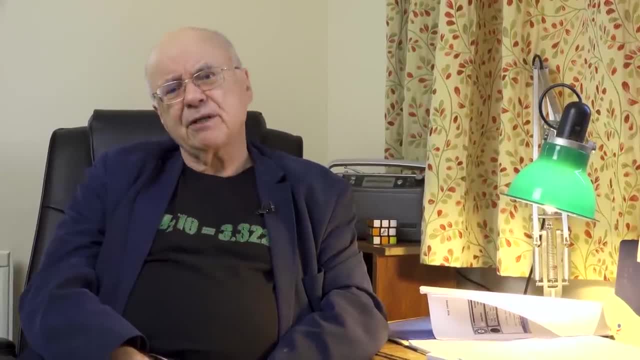 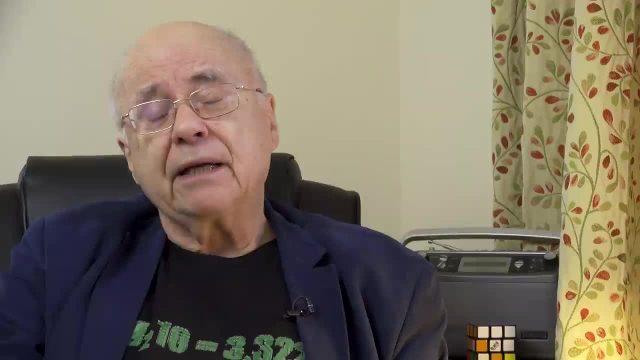 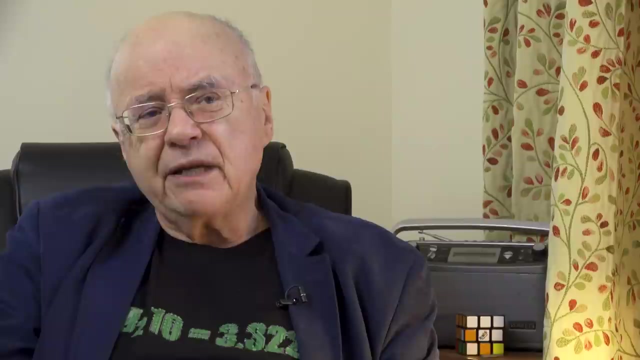 that community, I think at age 35.. Maybe slightly younger, Unbelievably young. He'd hardly been at Princeton a year or two as an ordinary mathematics professor. Everybody thought this is a truly phenomenal person. He reminded many people of absolute superstars like Newton Gauss. 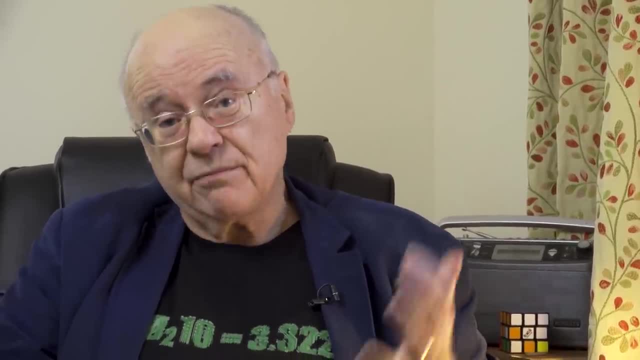 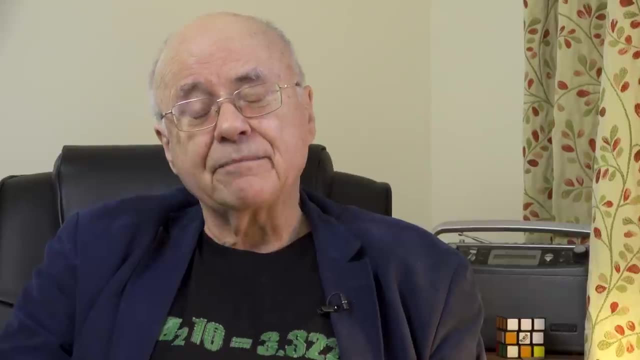 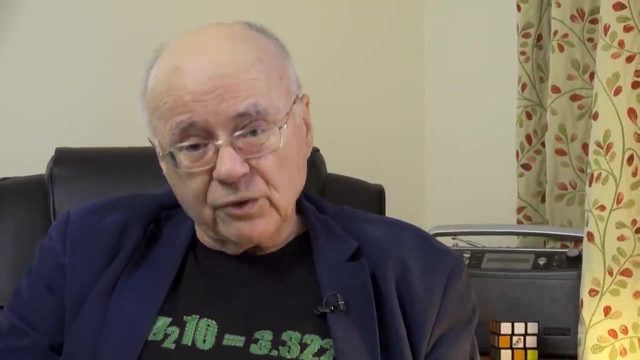 Euler, Einstein, Hilbert himself. Even at mid early to mid thirties, they could see that potential in him there. So yes, Turing visits Princeton in 1938, worked with Alonzo Church, but also, of course. 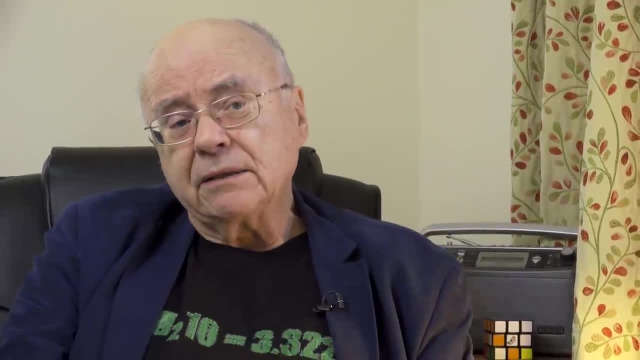 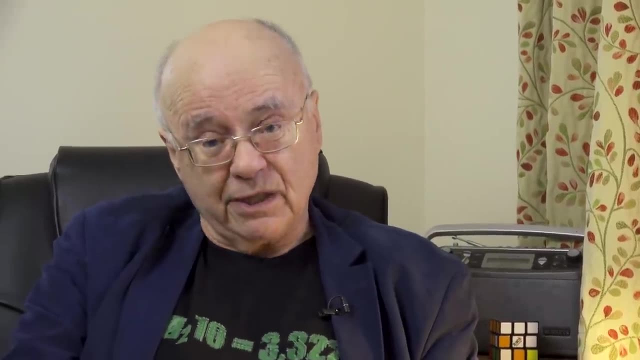 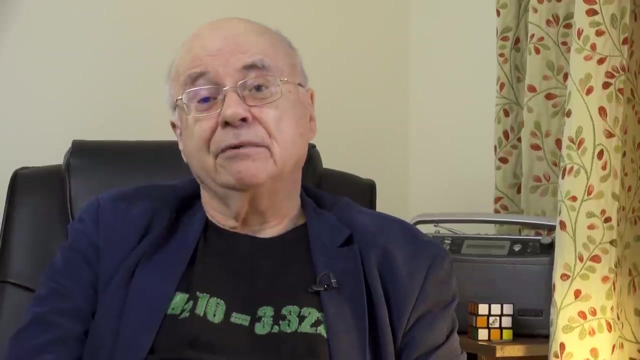 had frequent interactions at seminars with Von Neumann And then became the big question, if you recall, for Alan Turing: Should I return to England and do my patriotic duty? According to Andrew Hodge's definitive biography of Turing, Turing's father was all for Turing staying in Princeton. 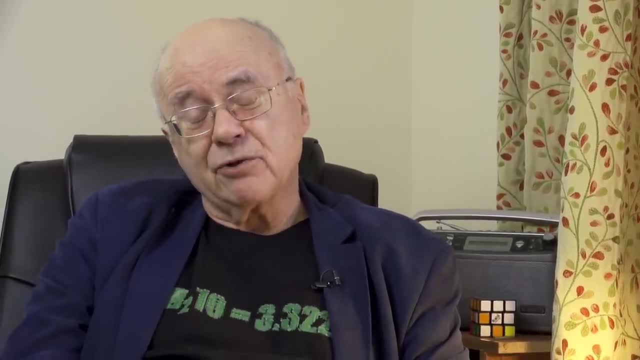 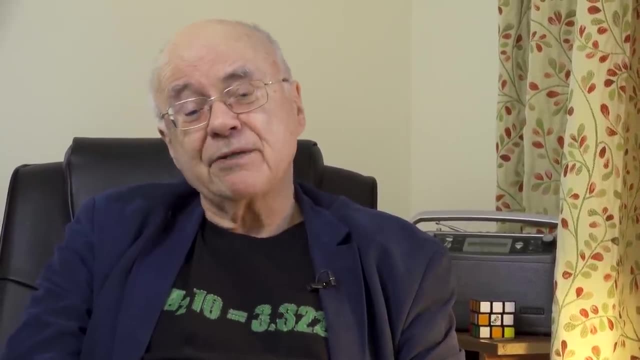 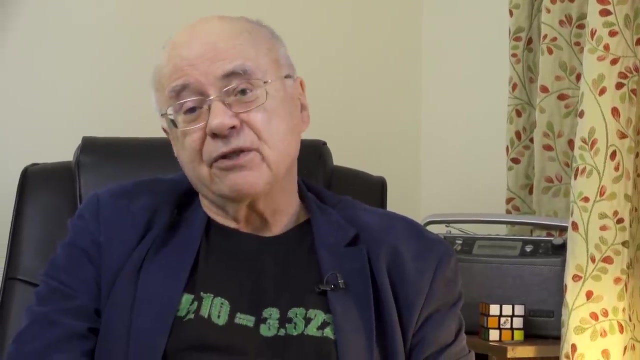 You know, keep out the war, get a prestigious mathematic job. And that was underlined by the fact that von Neumann offered Turing a job. He basically said: Turing, would you like to be my research assistant at the Institute for Advanced Studies? Now Turing could see straight away. that would just make you as a 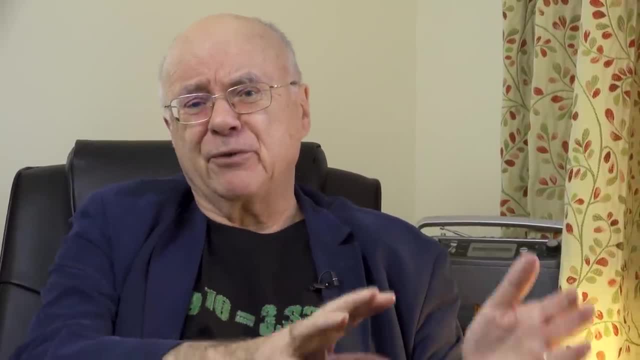 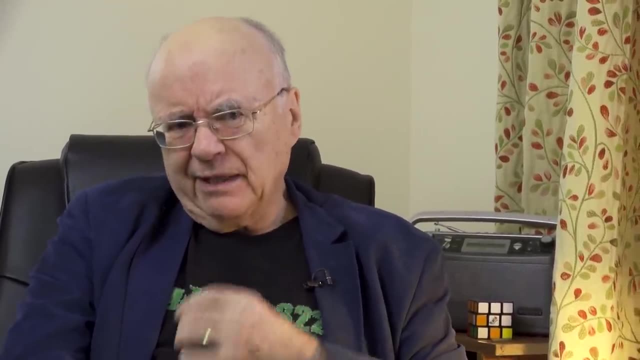 mathematician. you were invited by the great von Neumann to be his research assistant at IAS. Only problem was, I think, first of all I think Alan Turing did feel a certain patriotism in wanting to come home and do his bit. There was. 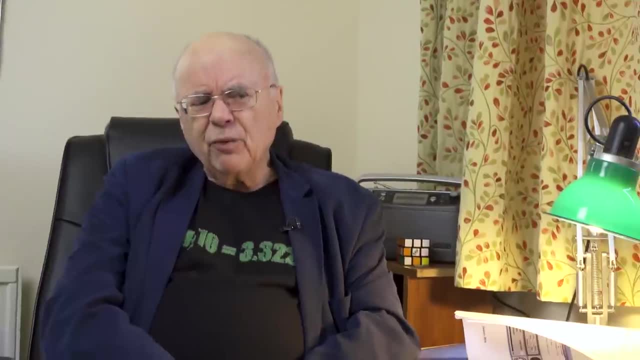 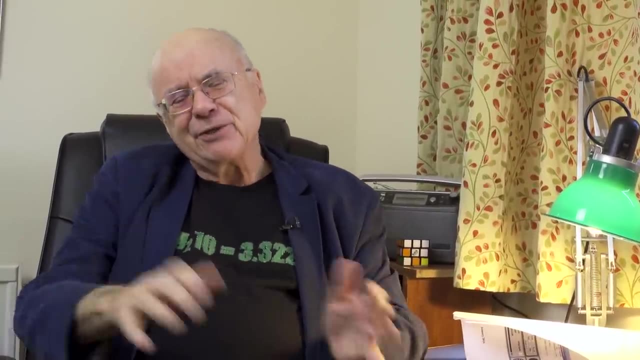 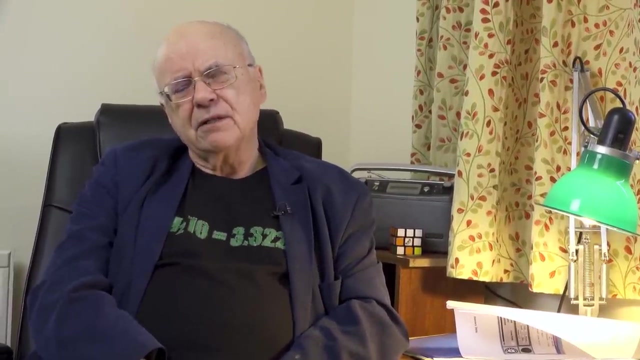 also the worry that at that time von Neumann had not properly got into computing, He had not turned his considerable talents to considering it, And for the research assistantship he wanted Alan Turing to do quantum mechanics. another of von Neumann's great love, And I don't think 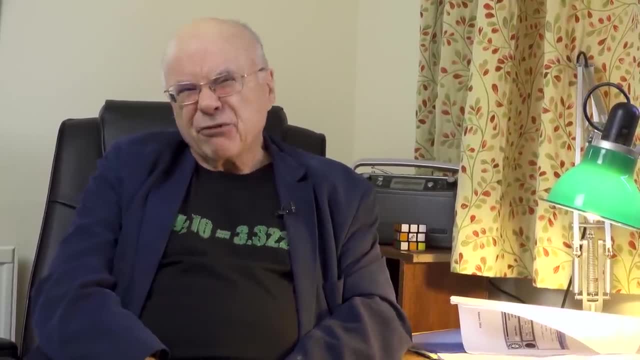 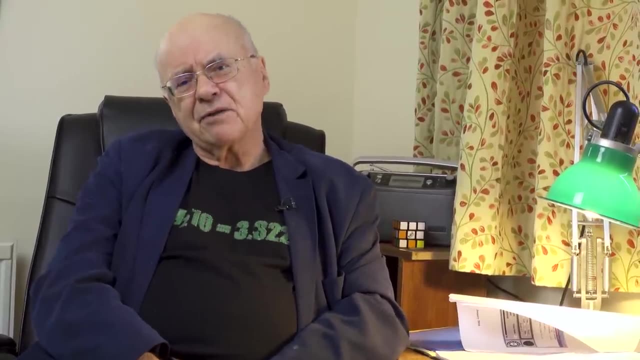 Turing was keen on that because he knew from experience at Cambridge, where he tried doing mathematical physics, it really wasn't his arena at all. So he politely declined with great thanks, came back to England And the rest, if you like. 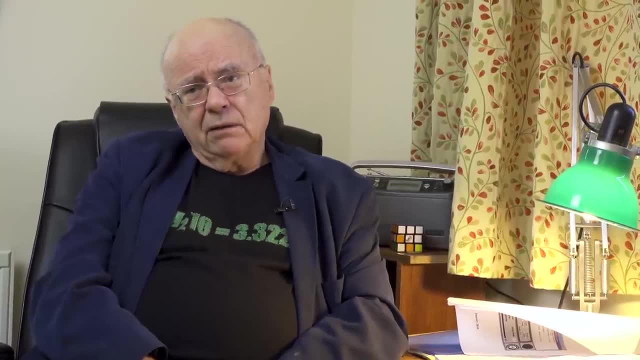 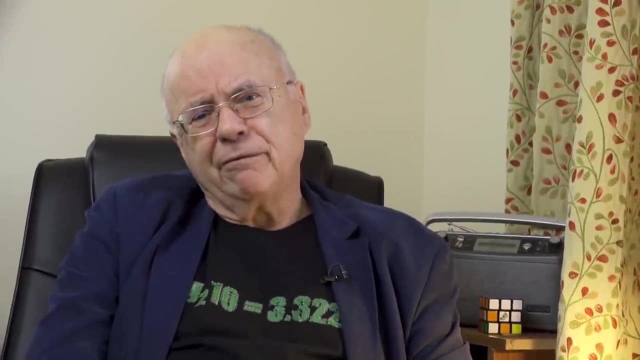 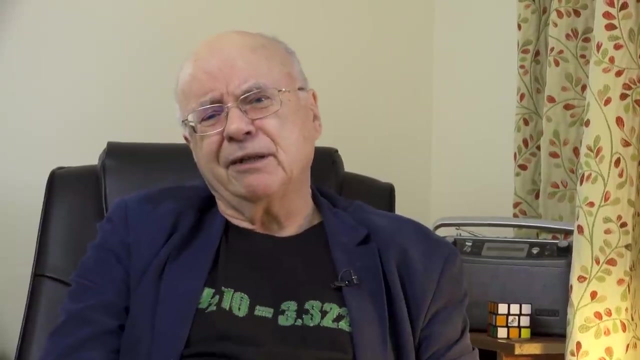 is more or less history. Now there's Johnny, as he'd now become Johann von Neumann, speaker of four or five languages, including Italian and English once he'd transferred from Göttingen to Princeton, wanted to become the all-American genius. So he was. on more formal occasions, he was 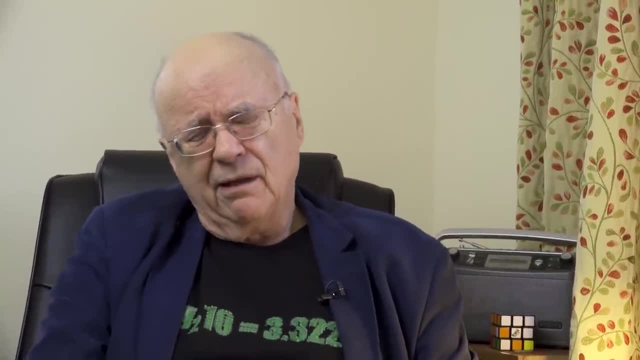 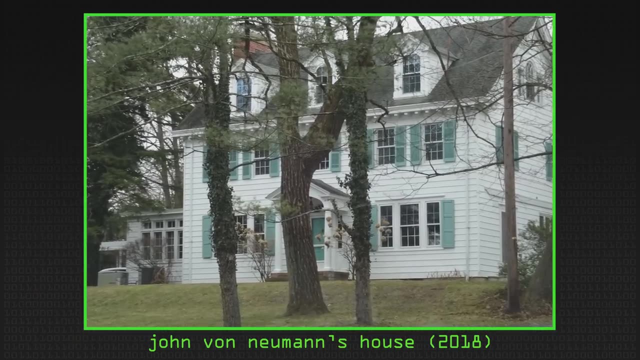 just John von Neumann, But to his friends he was Johnny. Oh, You can't exaggerate enough. I mean, his wife said he can count everything but calories. He was fond of food and drink. the champagne parties, the glitz, the glamour, the girlfriends- Good. 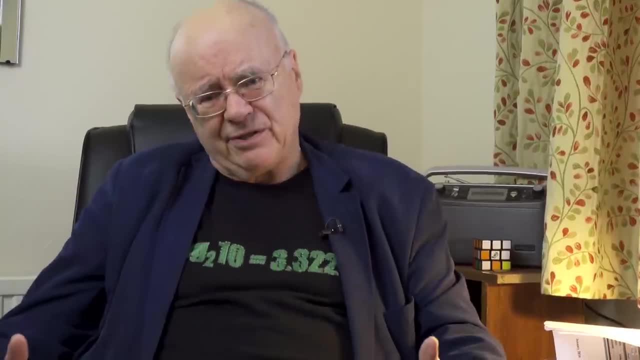 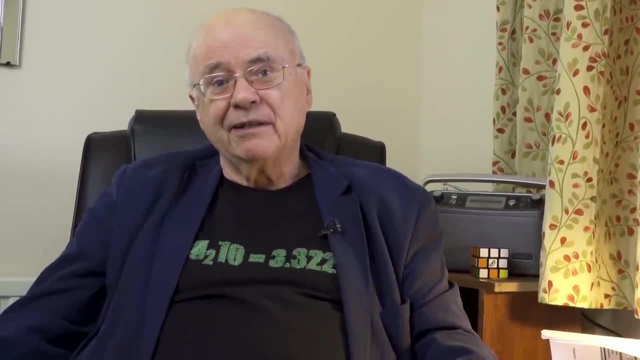 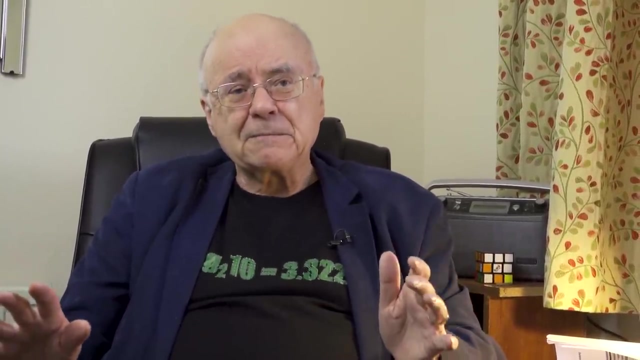 old Johnny. He absolutely was the antithesis of the shy mathematician. He was all-encompassing, and everybody who met him was just stunned by how he could see his way through problems in no time flat and just do impossible things. And so he was there in a very, very nice. 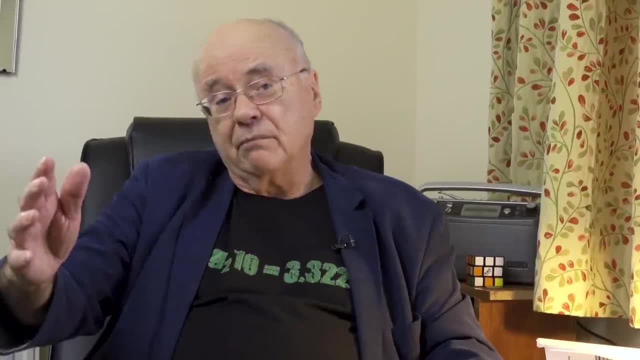 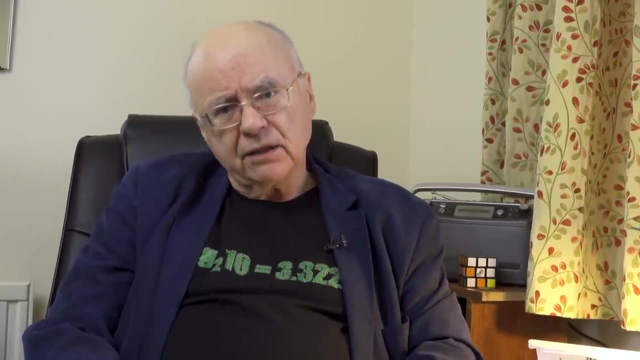 position in the Institute for Advanced Studies even before the Americans joined the war, But he stayed there throughout the war. But, being who he was, he was endlessly in demand be a consultant And, most famously, along with people like J Robert Oppenheimer, he 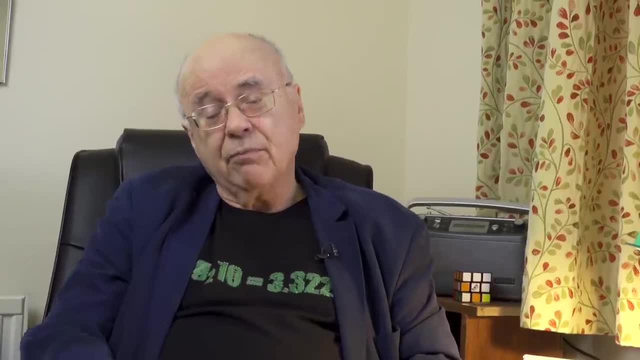 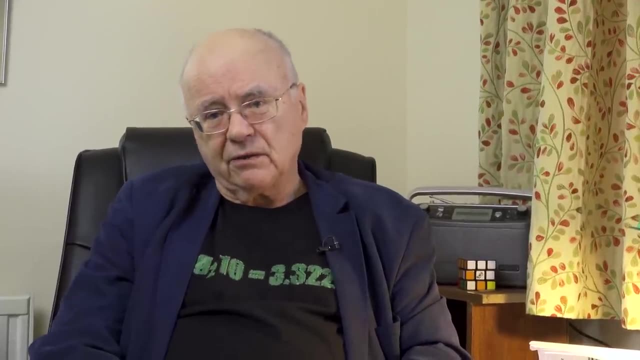 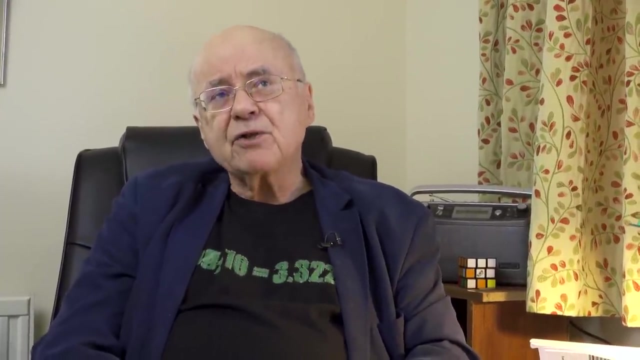 was one of the consultants employed on the Manhattan Project, the atomic bomb and the hydrogen bomb, But he was used by the Army, the US Navy, the Air Force. Everybody wanted Johnny as their consultant And this even included, as the war developed, the fact that one of the earliest computers which we have 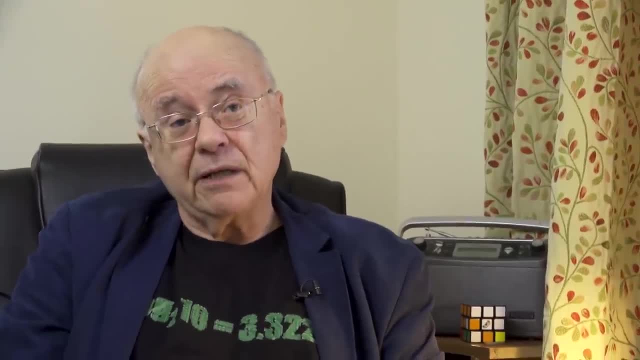 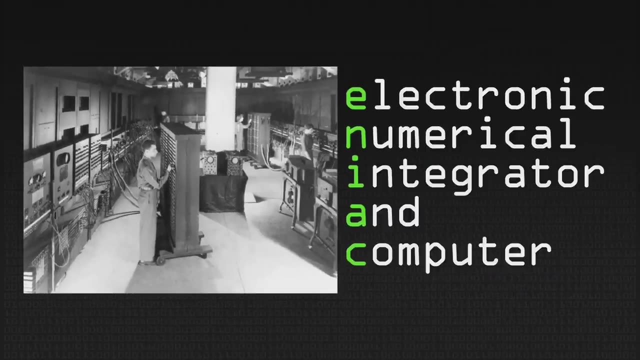 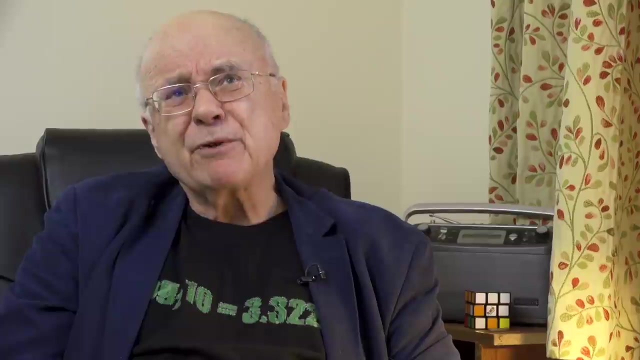 mentioned in a previous video was University of Pennsylvania Moore School of Engineering. They helped develop the ENIAC which, if you remember, was a vacuum tube computer running on decimal arithmetic and initially devoted to gunnery trajectory calculations. It was a bit late in 1946 to be of direct 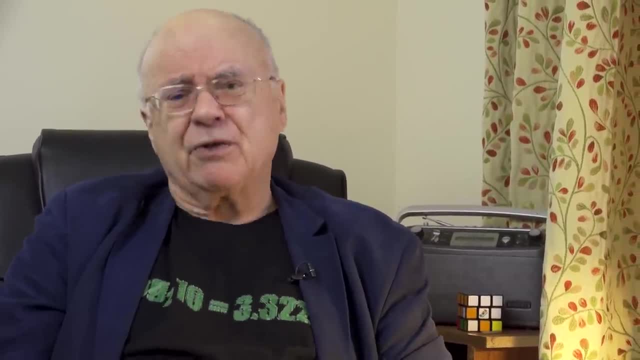 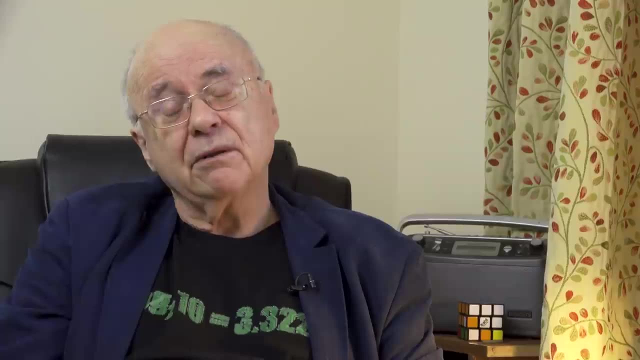 strategic use in gunnery. Actually, Johnny- who by this time, of course, was a consultant to the Moore School- devised a way, I think, to turn ENIAC into being a general-purpose computer, Although it wasn't a very efficient one, and I 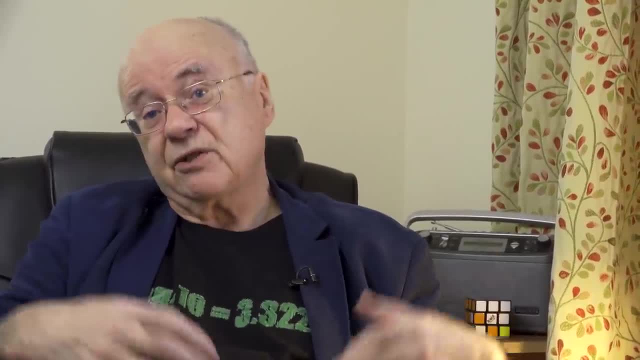 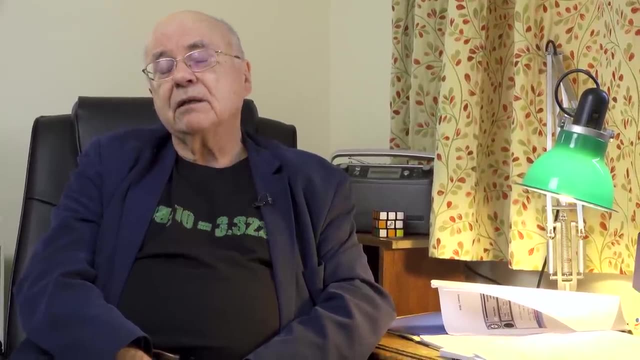 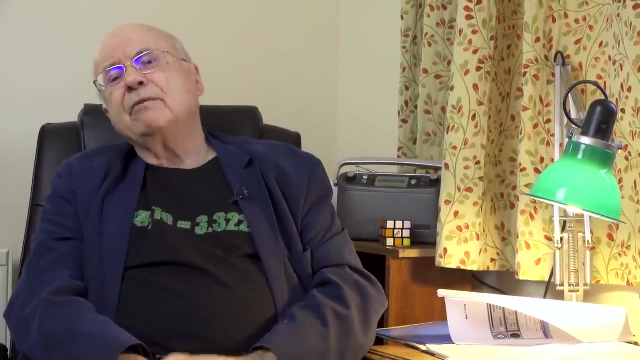 believe he used it for some reason- calculations relevant to the atomic bomb and all that kind of thing. The natural question arising with everybody at the end of the war went like this: We all know, or even though it's top secret, at Bletchley Park. we have heard gentle. 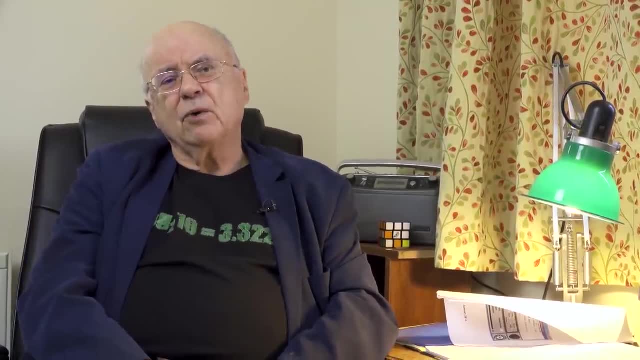 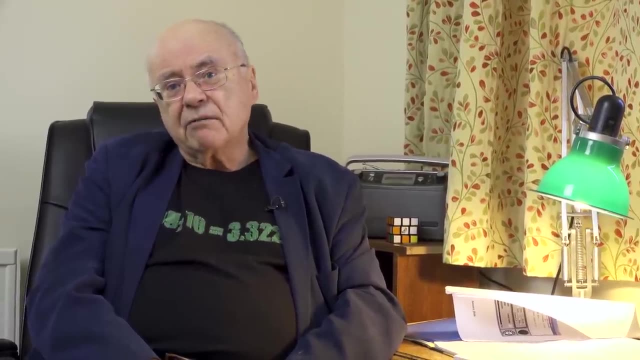 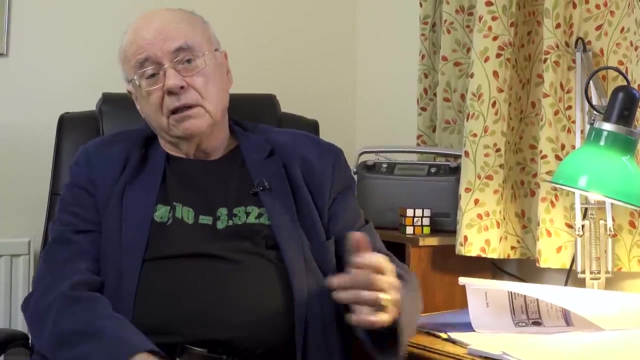 rumors that computers are being developed all over the place And you've always got to say: are they special purpose, Are they general purpose, Are they binary, Are they decimal, Are they fully electronic Or are they electromechanical? And literally there must have been at least a dozen machines. 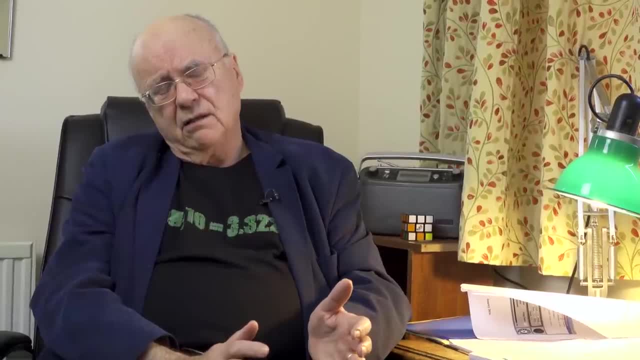 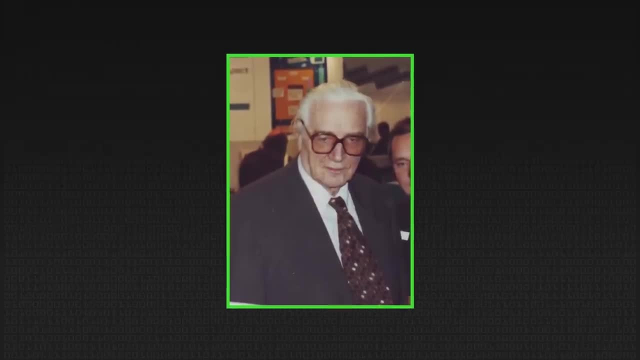 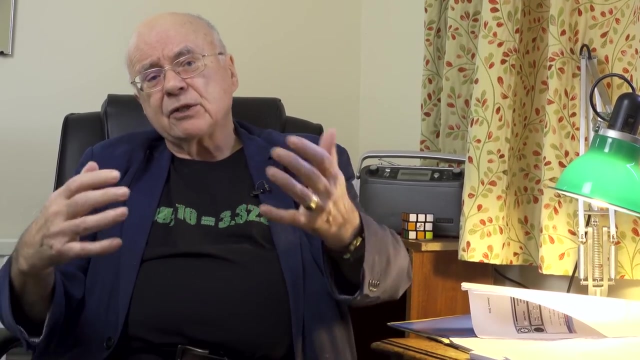 around that satisfied some of these criteria. If you ask Germans about who's the father of computing, they say Konrad Zusser. He developed electromechanical machines that were Turing, complete and calculated things, but they never got beyond electromechanical. You get into electronic. 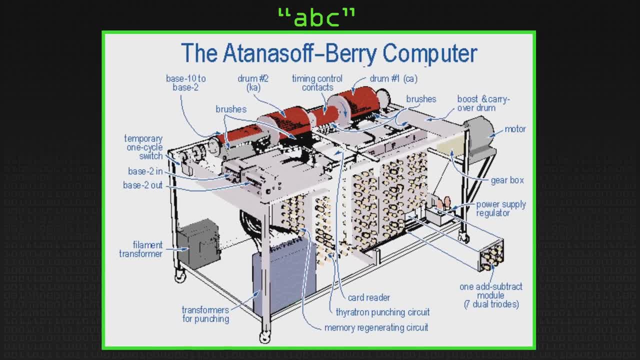 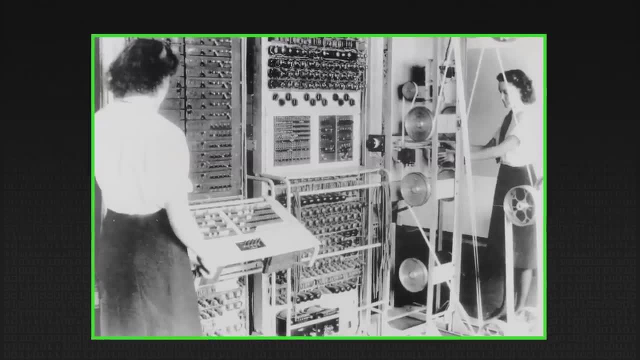 ones You get Atanasov & Beres electronic valve driven thing. Special purpose, though, could solve certain differential equations, And even Tommy Flowers and Colossus, we know. special purpose Can decrypt tiny traffic, Lorenz Cipher as it. 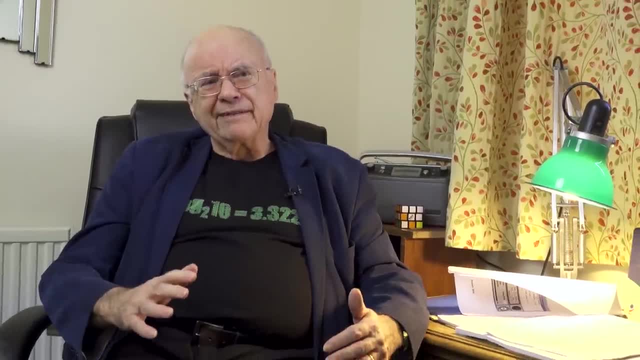 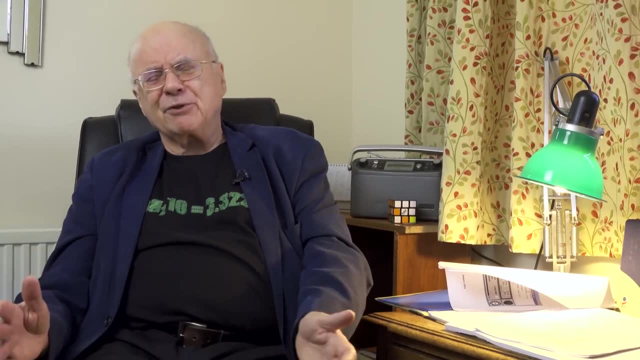 later become known as. So you've got everything happening: that if it's general purpose, it's not yet electronic. If it's special purpose, it is electronic, But we want it to be general purpose. So at the end of the war, it was the perfect time to. 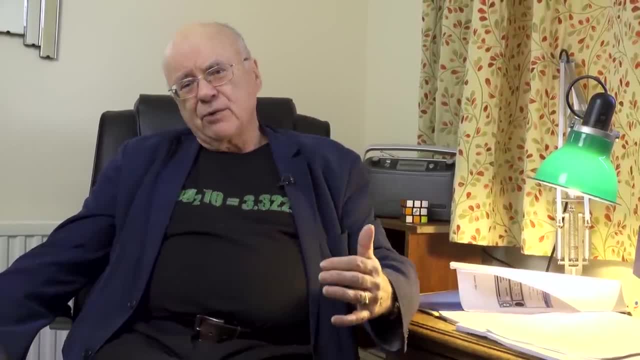 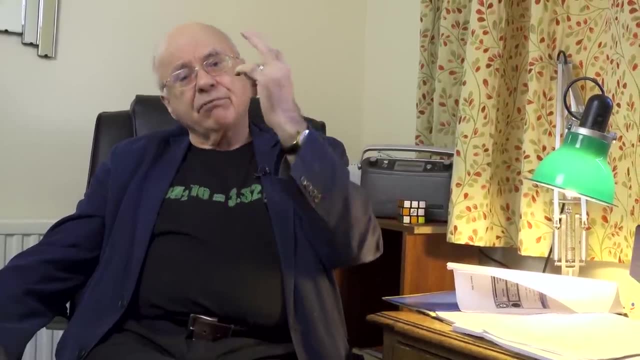 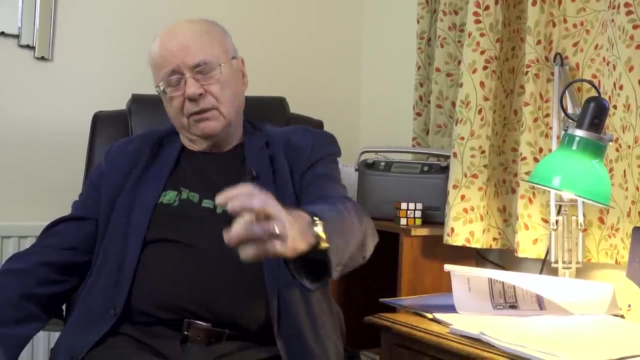 get everybody together and say: look, now that the war is over, we all want to find the way to do it correctly, To build general purpose- Probably binary-based because they're more reliable- All electronic digital computers. How do we do it? And who better to lead the charge and run a summer school and be 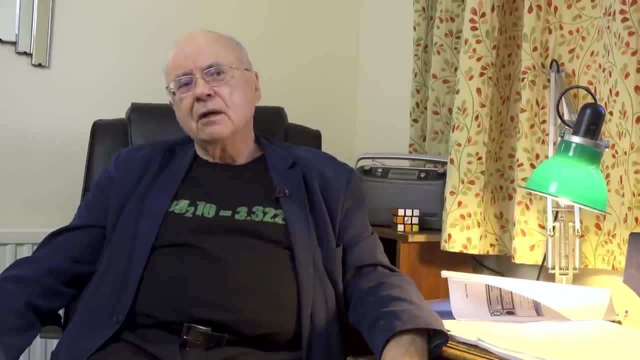 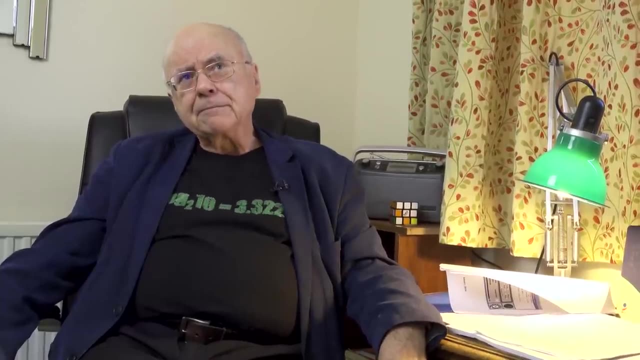 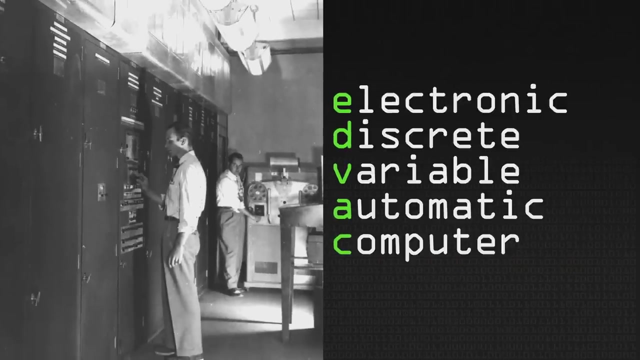 associated with it than Uncle Johnny, of course, And the Moore School at Pennsylvania, to their great credit, did this. they decided that the successor to ENIAC would be a thing called EDVAC. They said: yeah, it's gonna take us three or four years to do this, But in the meantime,